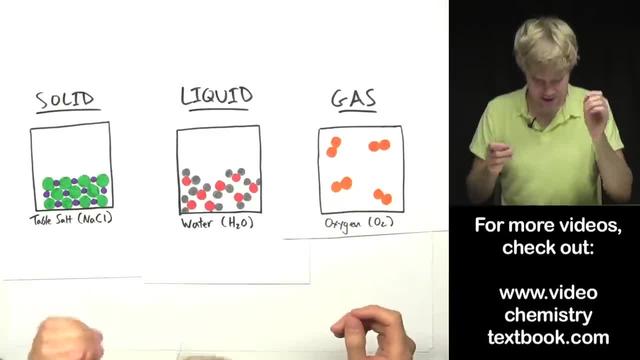 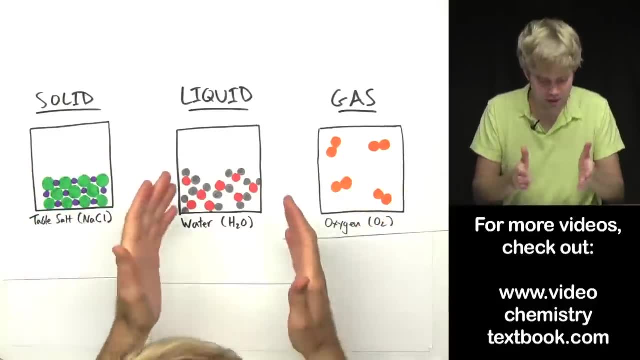 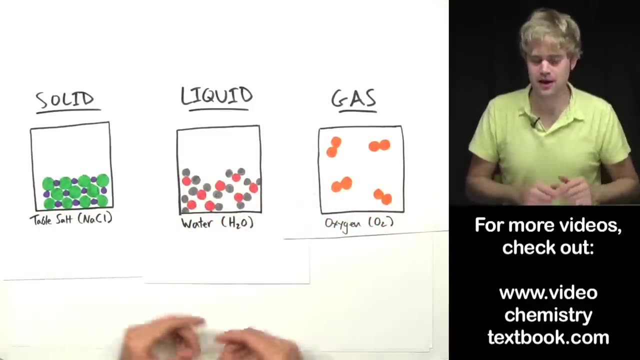 we could take these three things and zoom in zillions and zillions and zillions of times. If we could look at these closely enough, we'd be able to see the atoms, these little building blocks that make everything up. Now, atoms aren't really little colored circles. 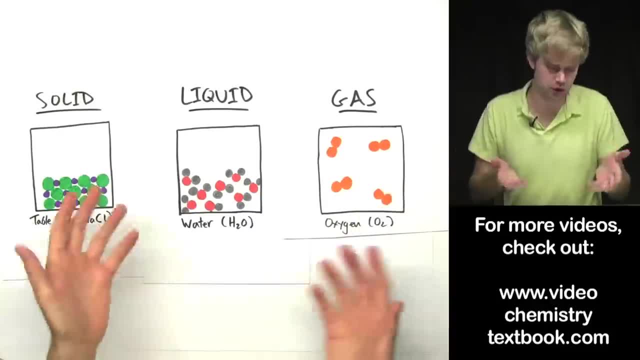 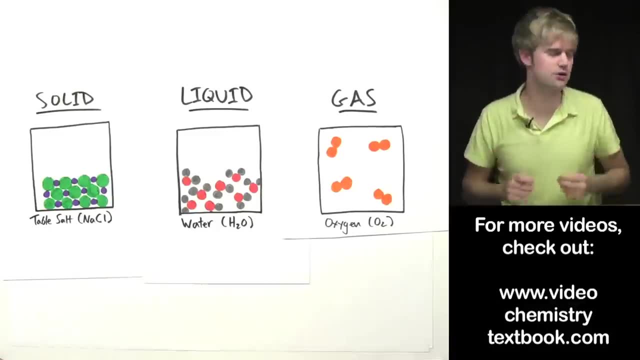 but it's a good way to think about them and it's the way we'll usually draw them when we're learning about this stuff. Atoms are super tiny. They are so tiny it can be really hard to see. You'll have to wrap your head around how tiny they are. Here is something that might 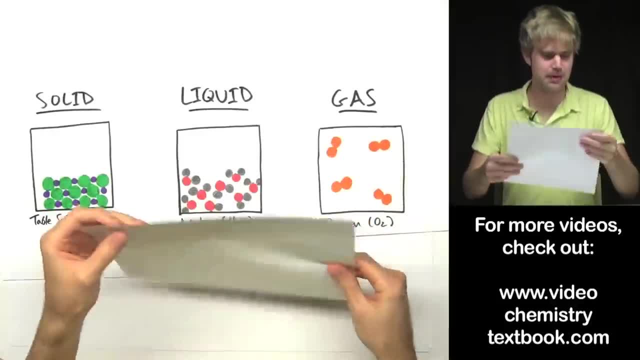 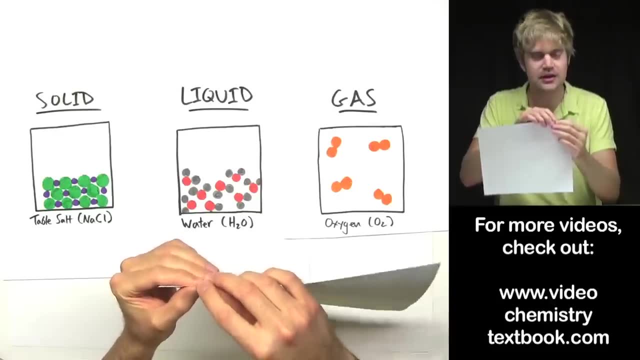 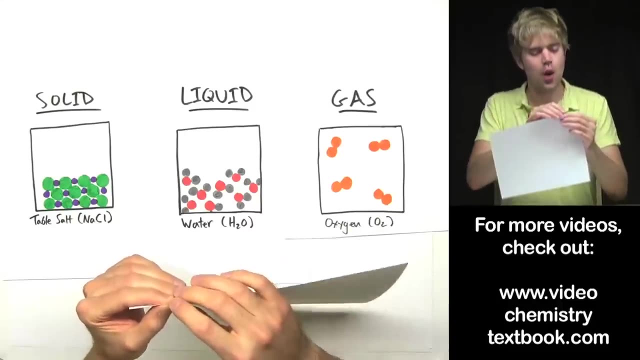 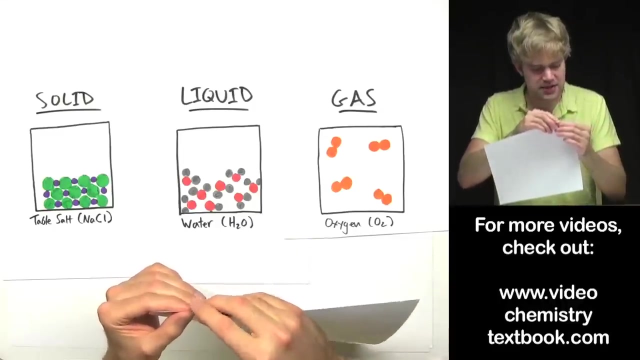 help you think about this. Take a piece of paper. Look at how wide it is here. All right, This is so incredibly thin. Now, atoms are so small that it would take one million atoms lined up next to each other in a row to be as thick as this tiny atom. 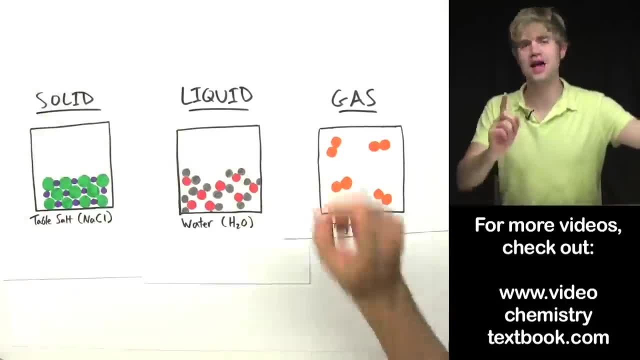 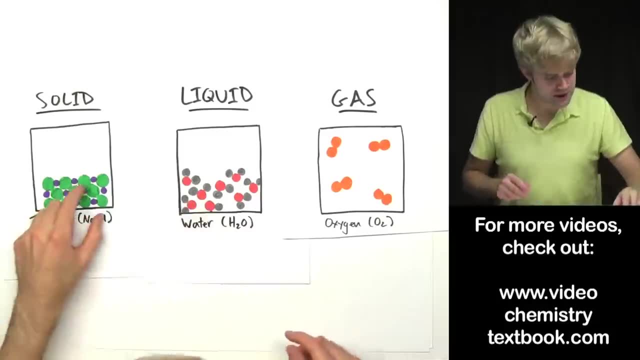 This is a tiny width of paper. That's how small atoms are. Now what I want to do now is look even closer at an atom. Let's take one of these atoms here and zoom in even more so we can see what's inside of it. 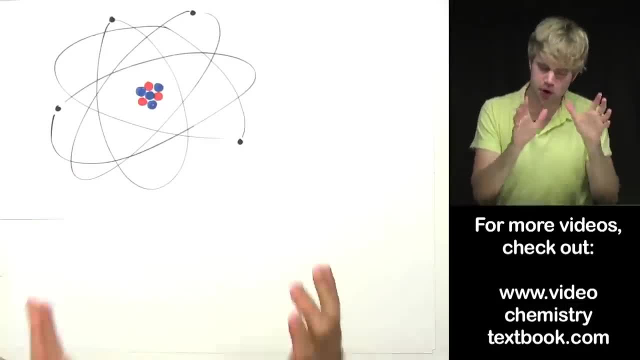 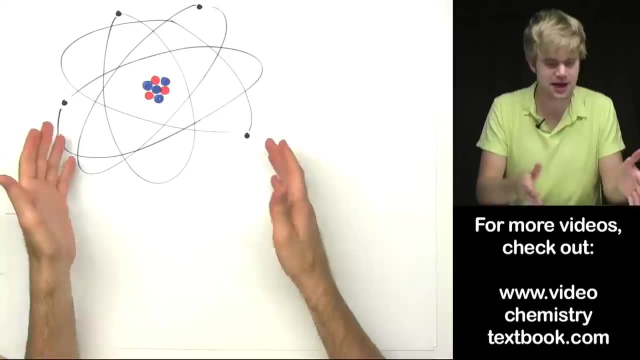 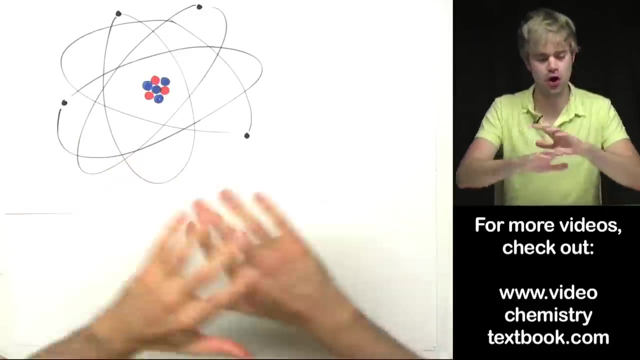 Here's a magnified view of one atom. It's not a perfect representation of exactly what an atom would look like, but it's close enough for right now. And check this out. The atom itself is made up of even smaller atoms, Even smaller things, Right, So that we said atoms are like the building block for all. 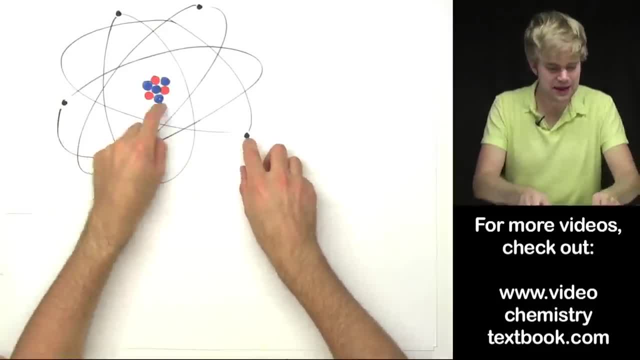 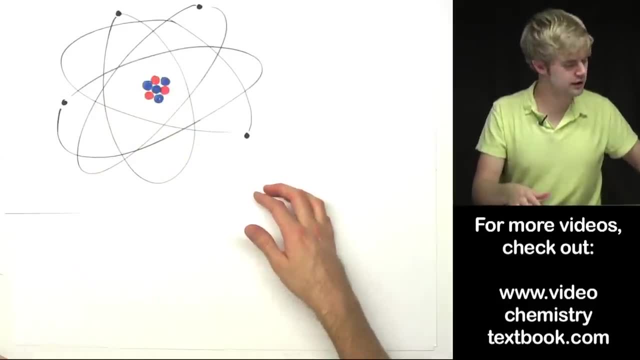 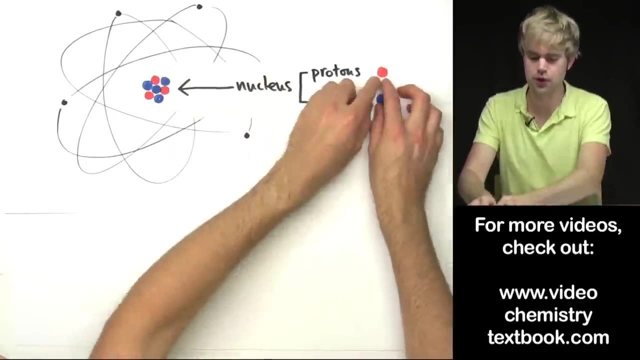 of stuff. but then if you look at an atom, it has even smaller building blocks that make it up. So in the center of the atom is something called the nucleus, And the nucleus is made up of two tiny particles. There are protons, which I've drawn as red circles here, and 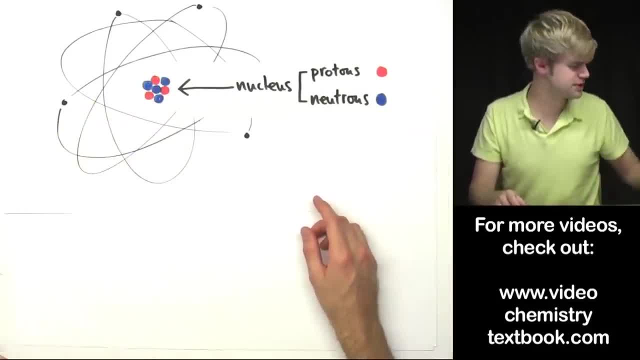 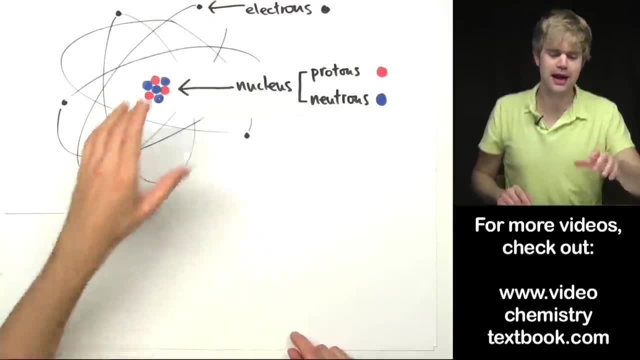 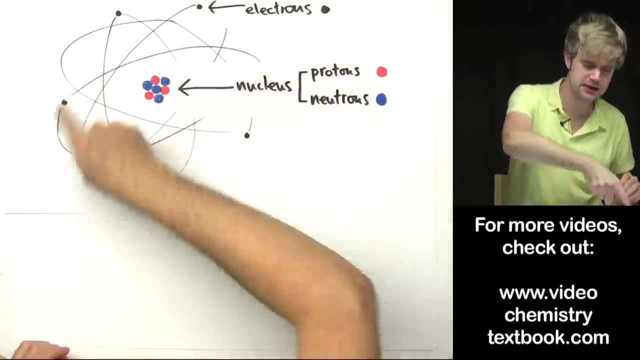 then there are neutrons, which I've drawn as blue circles. Nucleus is here in the middle of the atom, And then on the outside of the atom there are these little black circles that I'm using to represent electrons. The electrons you'll see are connected to these. 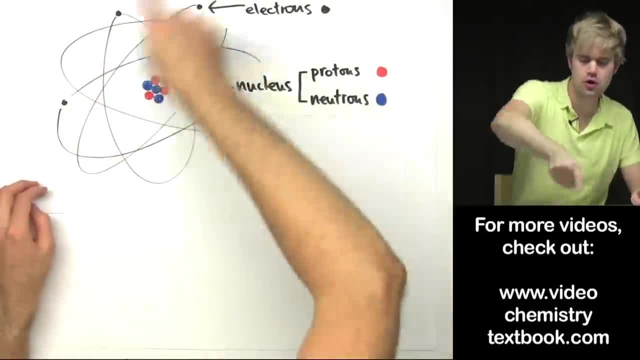 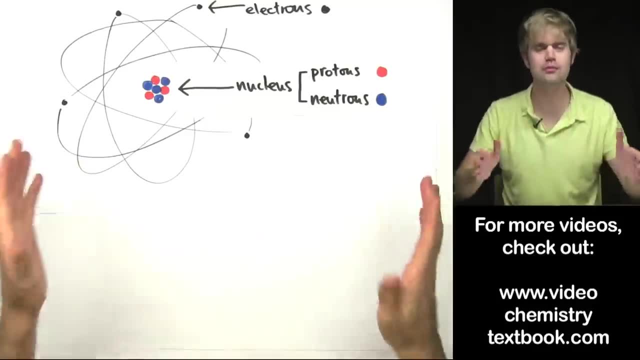 sort of oval paths, and I've drawn these in to show that the electrons are constantly moving. They're flying around the outside of the atom at an incredibly high speed, Whereas the nucleus stays solid here, right in the middle. Subtitles by the Amaraorg community. 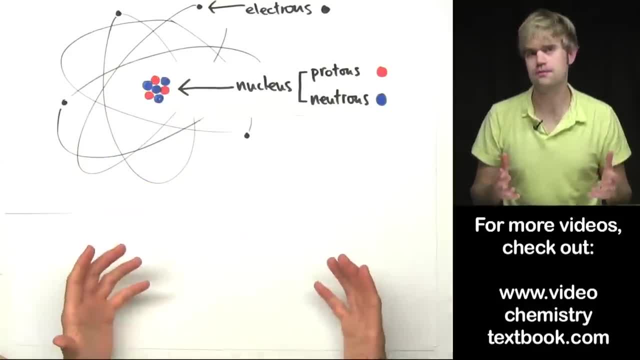 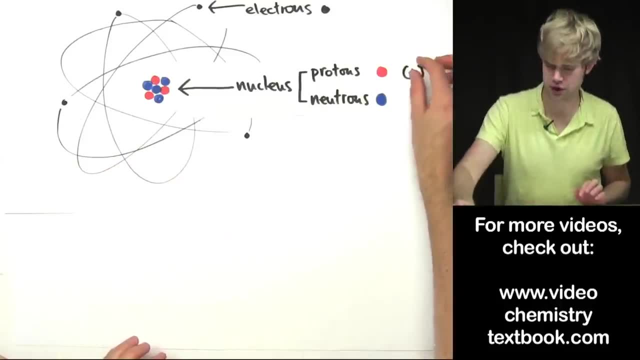 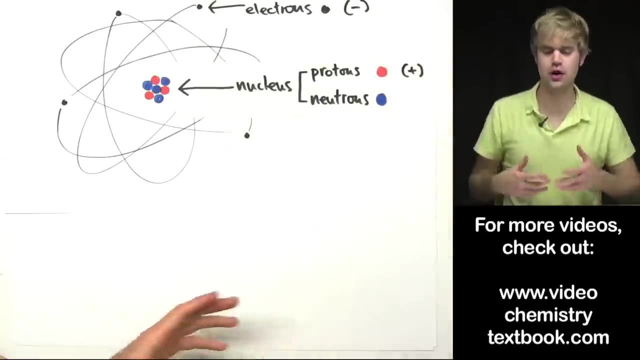 Now, electric charge is very important when we're talking about atoms for a number of reasons. Protons have a positive charge. A proton has a charge of 1+. Electrons, on the other hand, have a negative charge. One electron has a charge of 1-. Now neutrons, they don't. 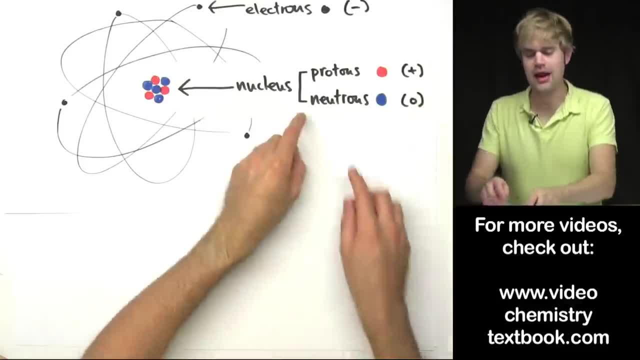 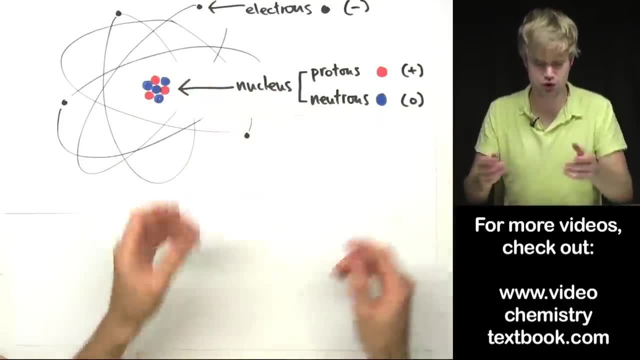 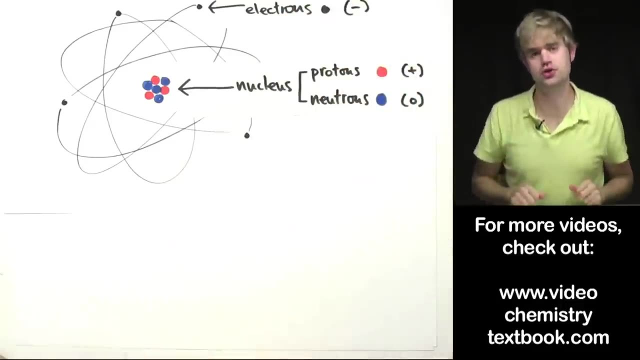 have an electric charge at all. They have a charge of zero, And neutral is a word that we use to refer to something that doesn't have a charge. Subtitles by the Amaraorg community. Now, positive and negative charges attract. Remember that Opposite charges attract, And 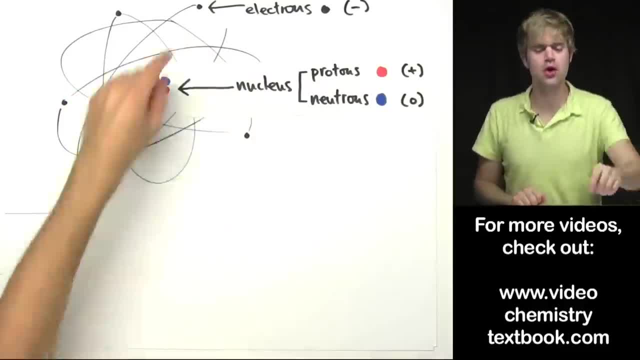 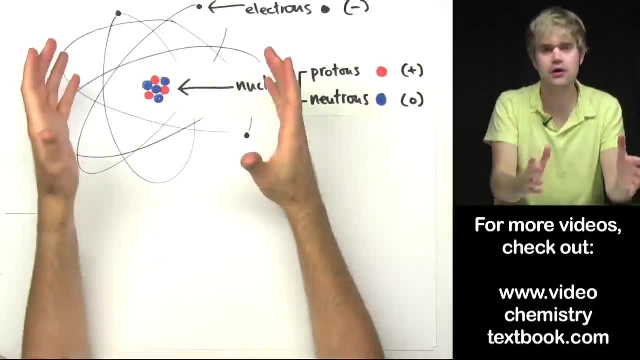 that has important consequences for how this atom works. We said that these electrons are flying around the outside of the atom. They're moving really fast, So why don't they just fly out into space? Well, the reason why is because the negatively charged electrons are. 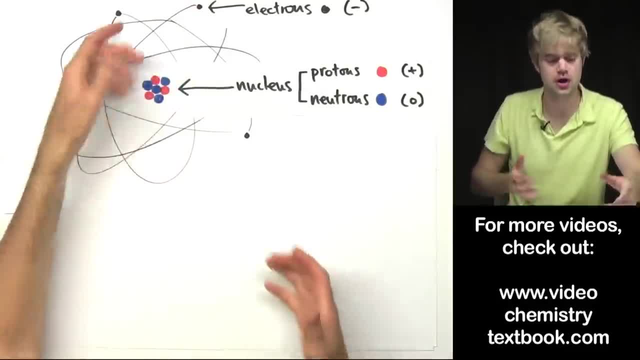 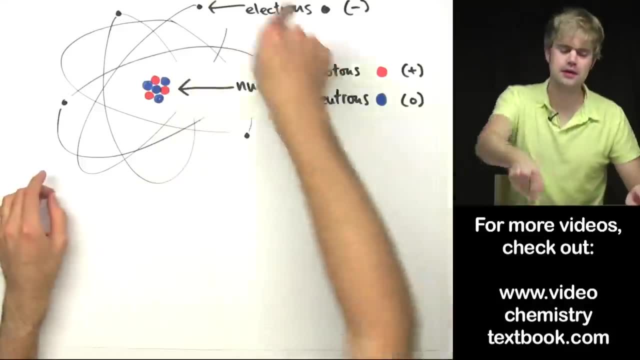 attracted to the positively charged protons. So the protons kind of pop out of the atom. They pull the electrons in. They keep them from just flying away. But the electrons are moving around so fast that they're not able to actually pull in here and actually 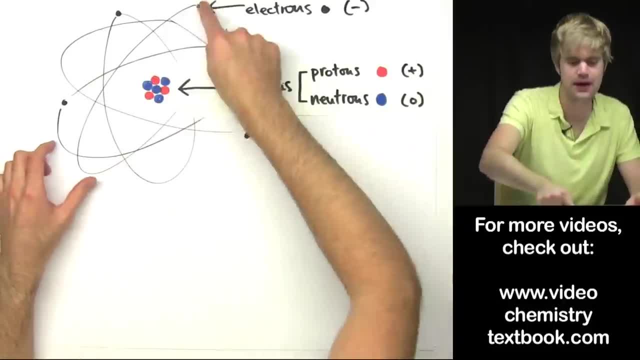 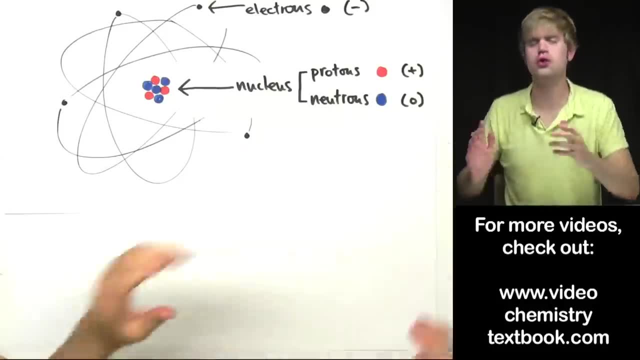 touch the protons. So that's why they keep staying on the outside and don't just crash in here and all touch the protons. Now sometimes people ask: well, neutrons, neutrons don't have a charge. Why are they important at all? Well, it seems that neutrons help keep all. 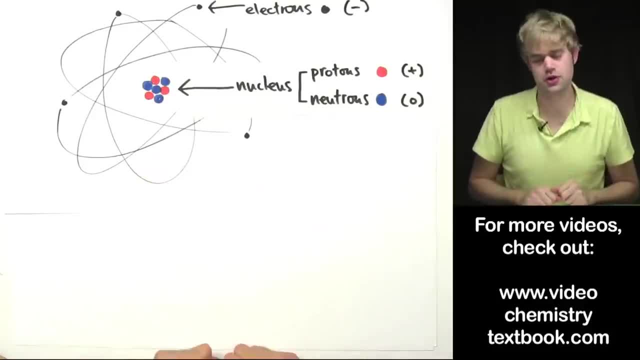 of the particles in the nucleus strongly connected to each other. Now, electrical charge is important. Something else that's important with atoms is what their mass is, how much they weigh. So in order to figure that out, we have to look at the mass of the various things that 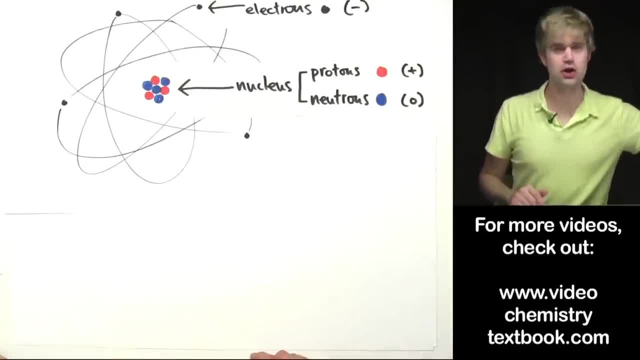 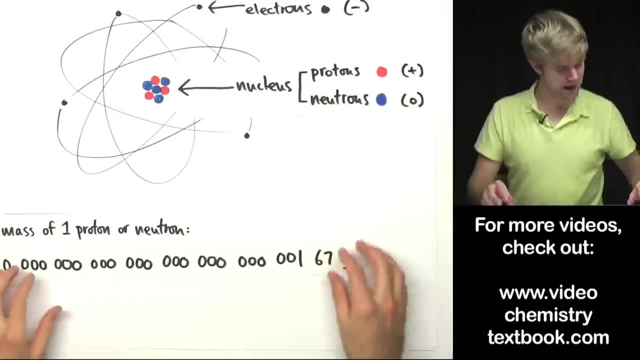 make up the atom. Now, a proton and a neutron are very, very similar in size and in mass, And they both weigh about this many grams. Look at what a tiny number this is. There's a decimal place all the way over here: This: 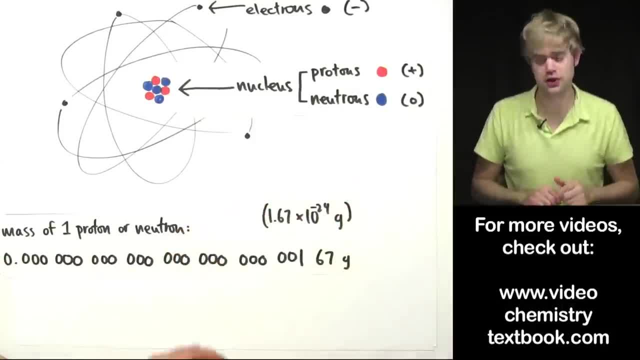 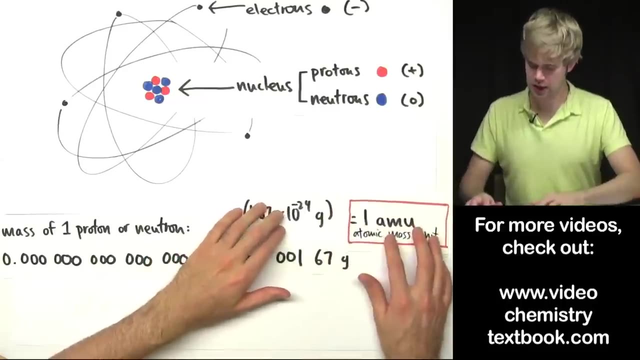 is a number that it's best to represent in scientific notation instead. But however you write this, it's a really tiny, unwieldy number. So scientists came up with another way to measure the mass of a proton or neutron, and that's using a unit called the AMU, the atomic mass. 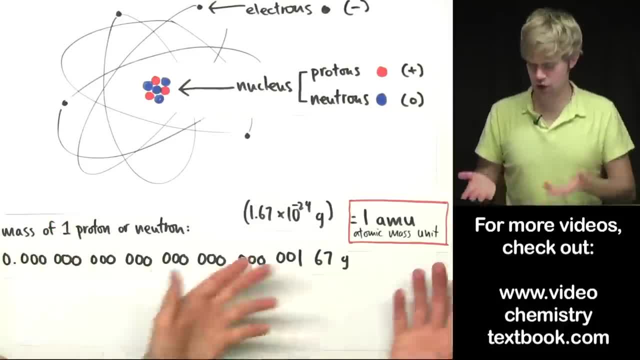 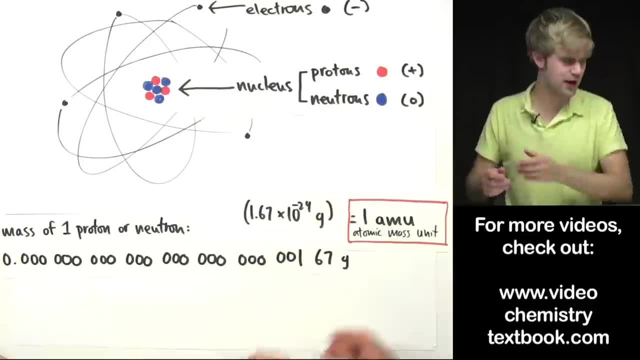 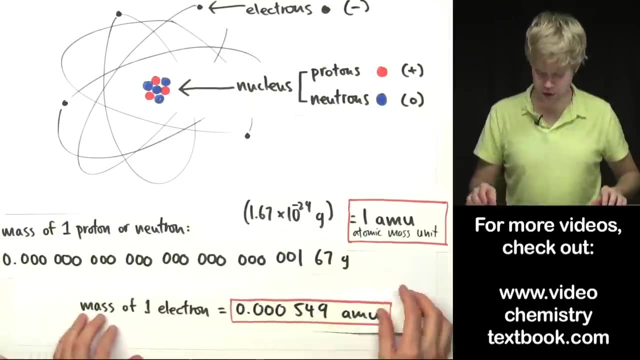 unit And they said: okay, one proton or one neutron weighs about one AMU. That's a lot easier to use than this measurement here. So proton or neutron weighs about one AMU. An electron, on the other hand, is much, much, much smaller than a proton or a neutron. 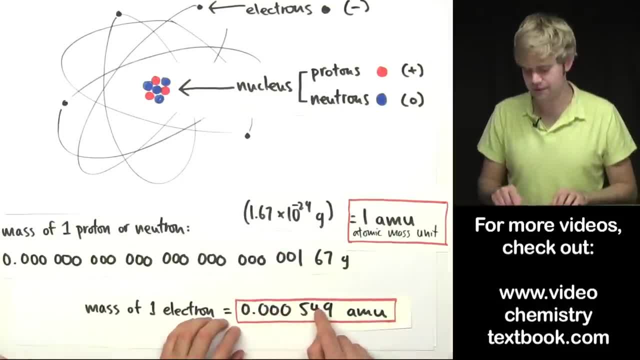 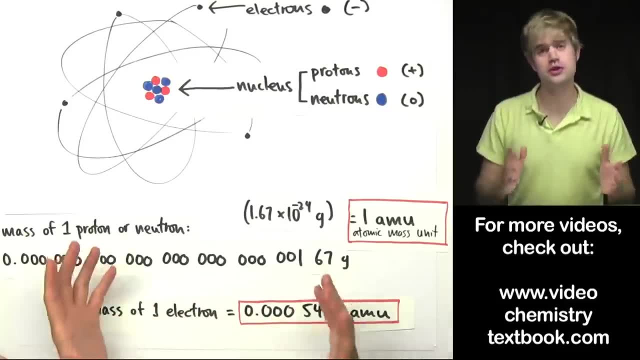 It weighs only 0.000549 AMU, so a tiny fraction of how much a proton or a neutron weighs. For this reason, when we're talking about the mass of atoms- which we'll talk about later on- we usually add up the proton and the neutron. 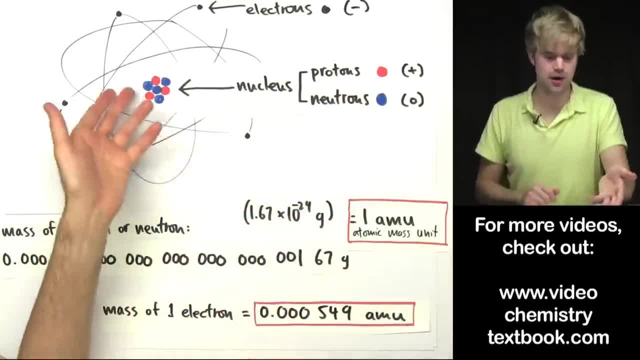 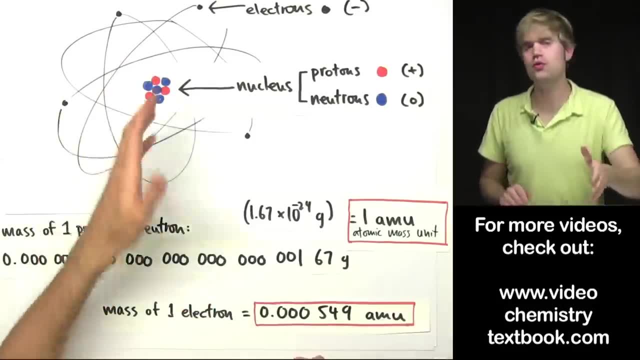 We add up protons and neutrons to find out how many AMUs the atom weighs, And then we usually don't even worry about the electrons at all, because they're just so tiny. They don't really have much of an influence on how much an atom weighs. It's like when you 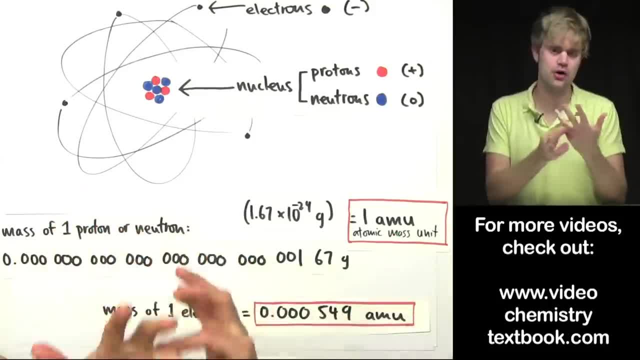 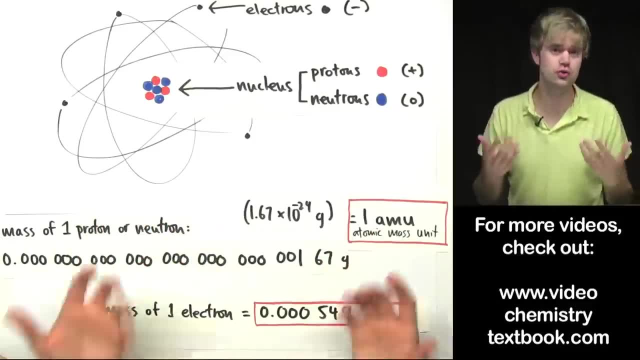 get on a scale to weigh yourself. you don't worry about the ring you're wearing or whether you're wearing a necklace or something, because those things are just so tiny. They weigh so little compared to how much you weigh that it doesn't really influence your weight. 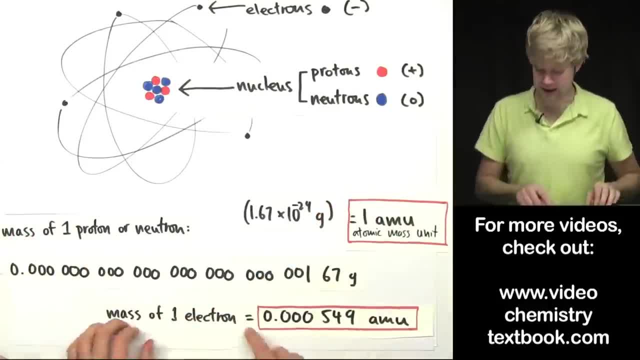 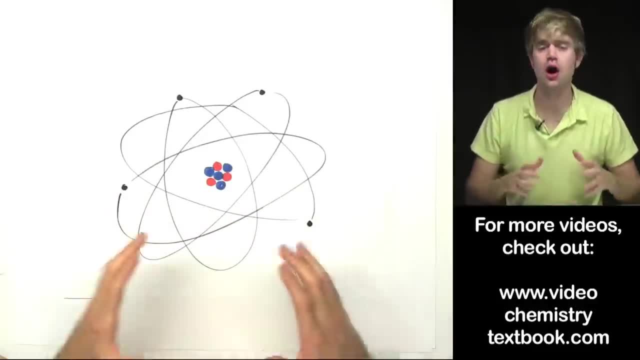 So protons and neutrons, one AMU And electrons- a tiny fraction of that. Now, I said that the atom, the way it's drawn here, isn't a perfect representation of what atoms would actually look like. We'll talk more about that later. but there are two things. 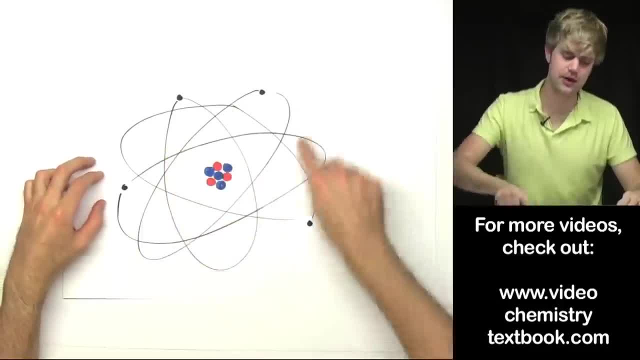 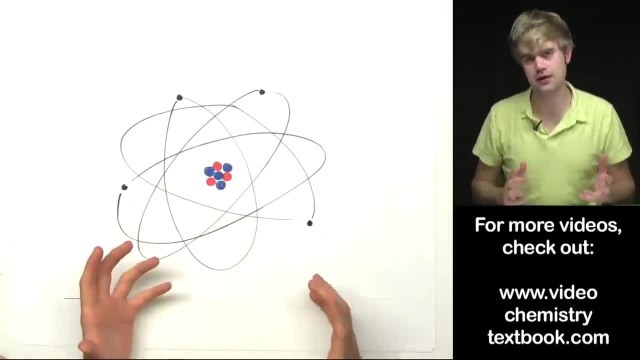 that I want to bring up for right now. The first is the electrons and how they move. This drawing might make you think that the electrons are spinning around in nice circles on the outside of the atom. That's actually not what happens. They're buzzing around much. 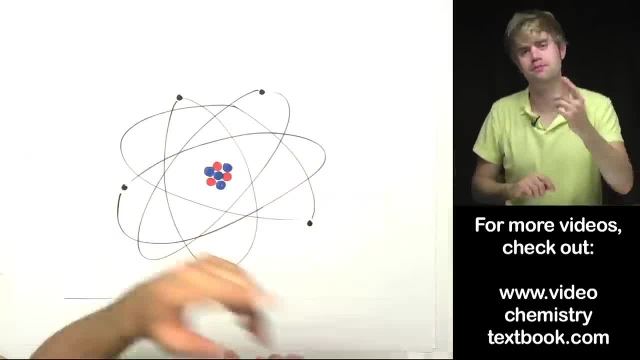 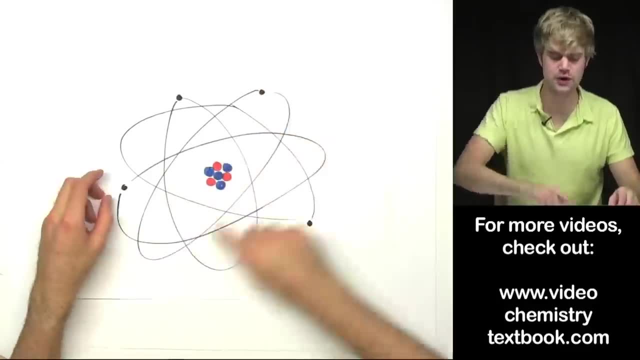 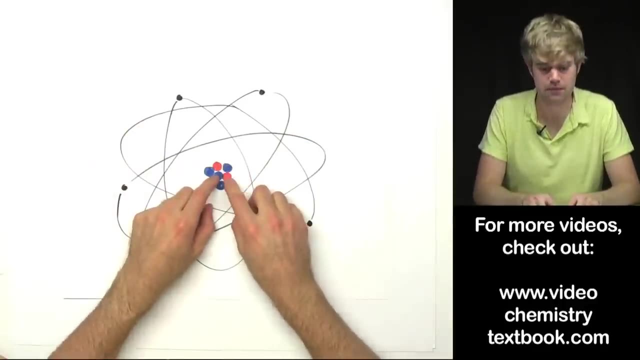 Kind of like hyperactive, flies all over the place. We'll talk more about that later. The second thing has to do with the size of the nucleus and how far the electrons are from it. If this were a real atom, blown up many, many times, and the nucleus were the size of a grape,